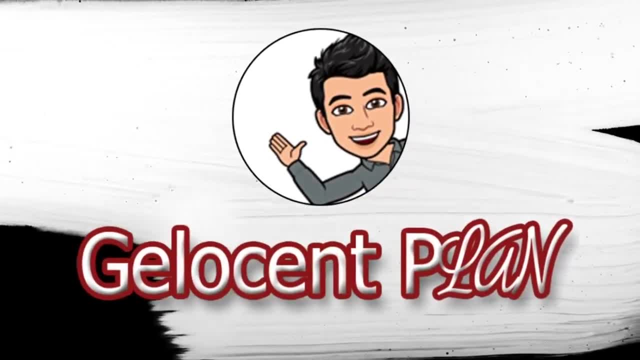 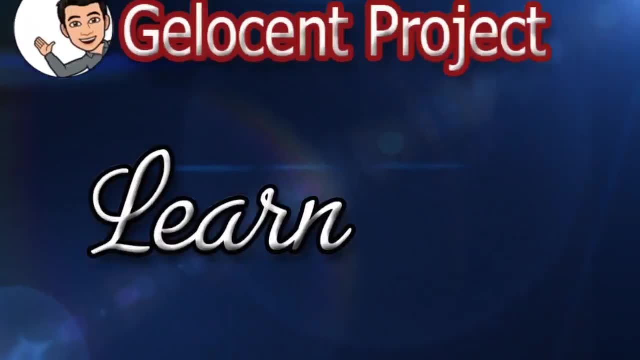 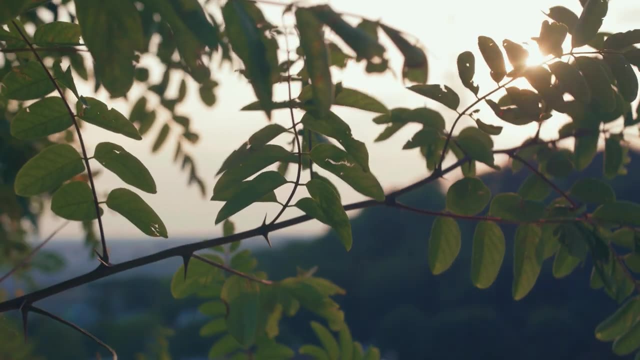 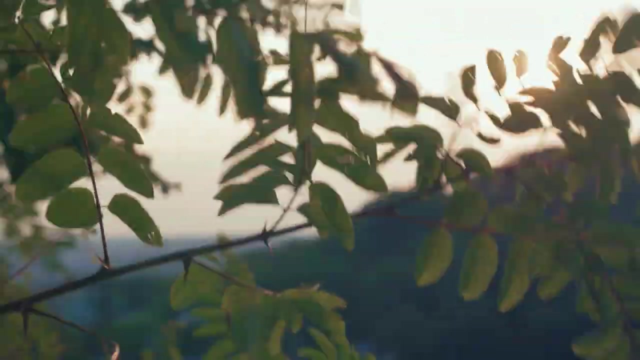 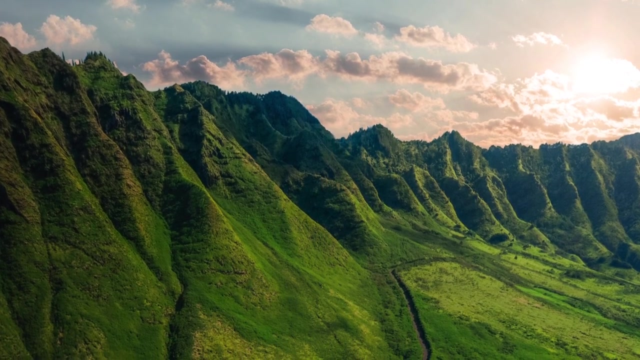 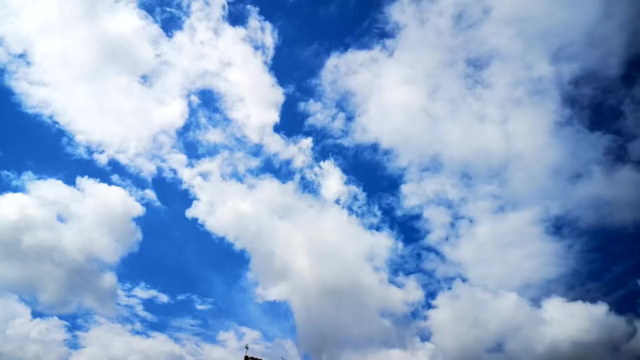 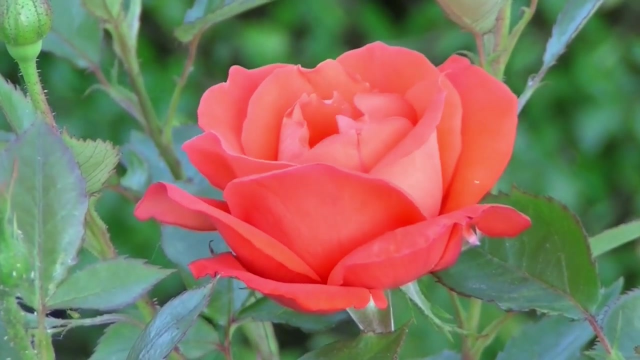 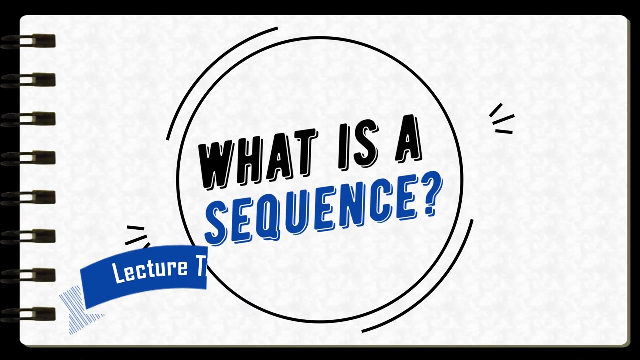 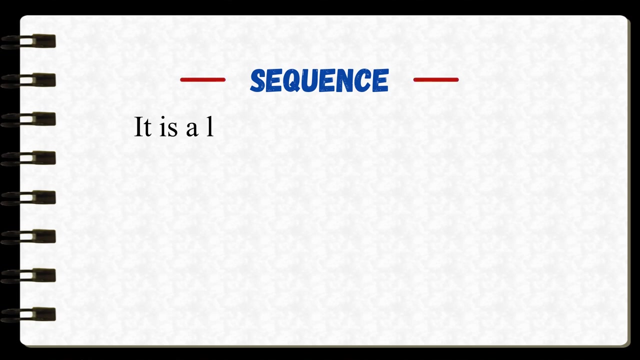 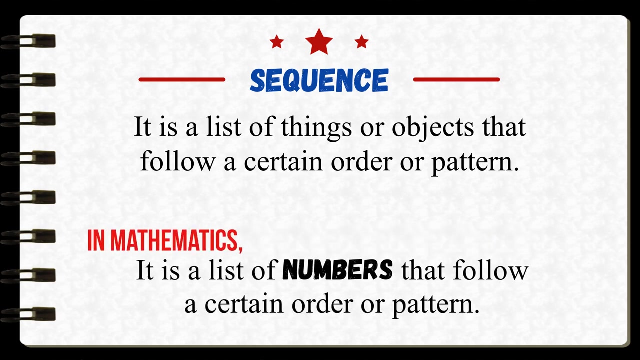 The beauty of nature Breathtaking, Simply amazing. What makes nature wonderful? This is because of the real-world patterns and sequences. So what is a sequence? Sequence is a list of things or objects that follow a certain order or pattern. In mathematics, it is a list of ordered numbers. 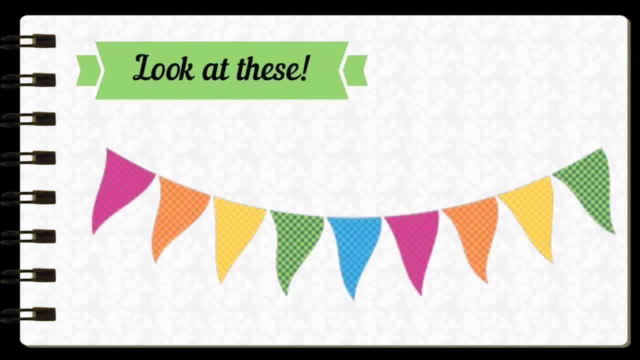 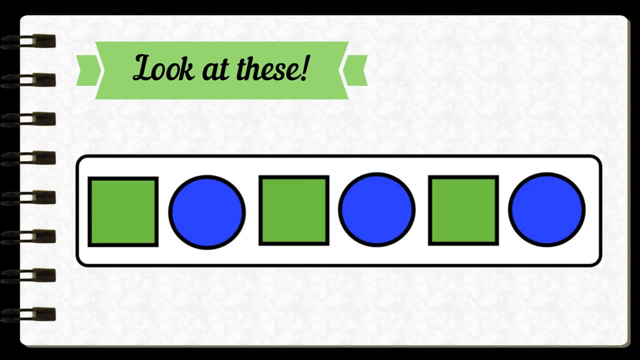 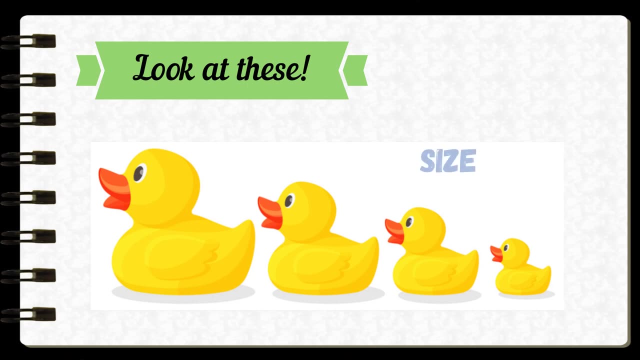 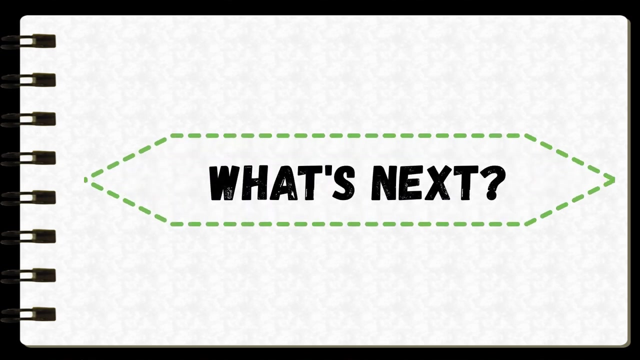 So let's take a look at these images. The pattern that is shown here is the color right In here. That's right the shape. How about? here? It is the size. Very nice, Nice. Now can you guess what's next in each sequence? 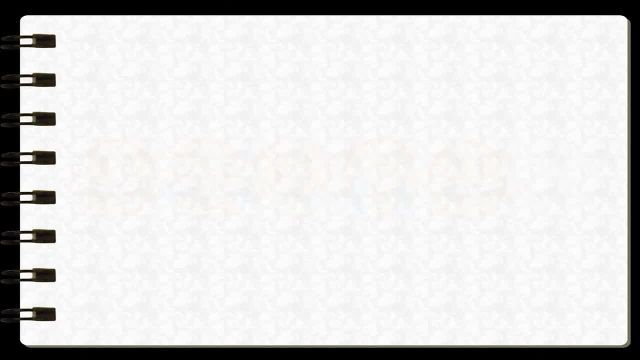 Inverted yellow triangle, A laughing emoji. Of course it's the letter J. Guess it. Yes, it's F. F for Friday. How about this? You can pause the video to make a guess. The correct answer is S. 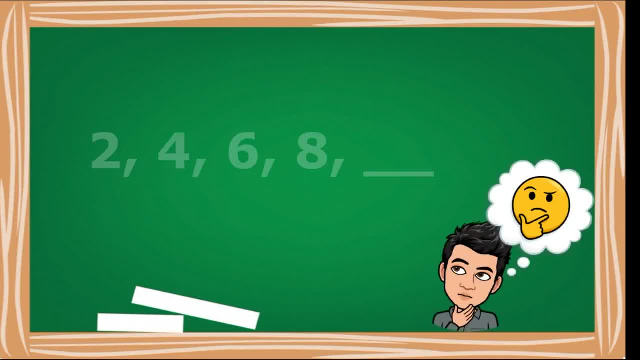 S for 6.. Interesting right. Let's try it with numbers. The missing number is 10.. The pattern Just add 2.. Next, the missing number is negative: 2.. The pattern Just subtract 3.. The missing number is 24.. 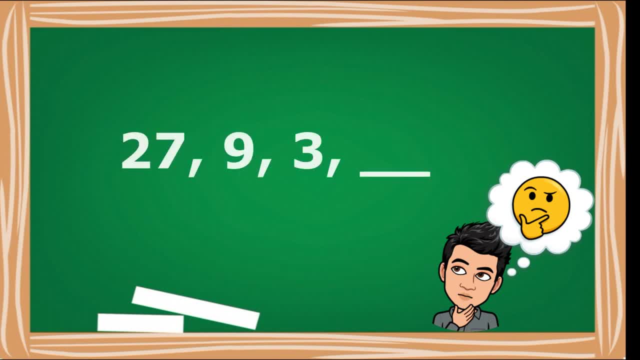 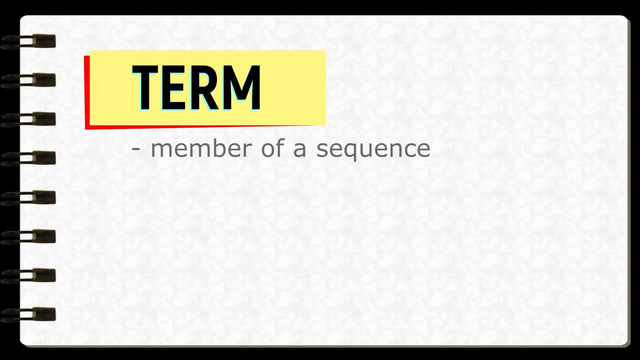 The pattern Multiply by 2.. The missing number is 1.. The pattern Divide by 3.. Very easy, right Now. each member of a sequence is called term. So the first member is the first term, The last member is the last term. 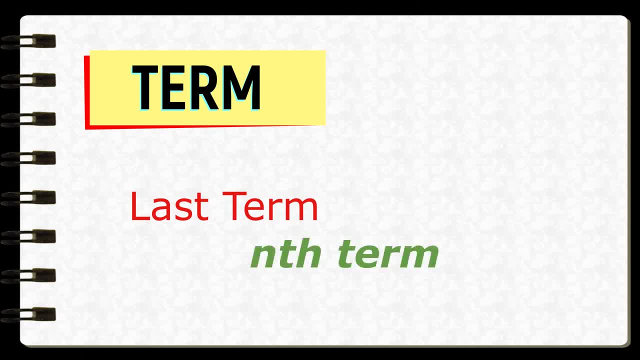 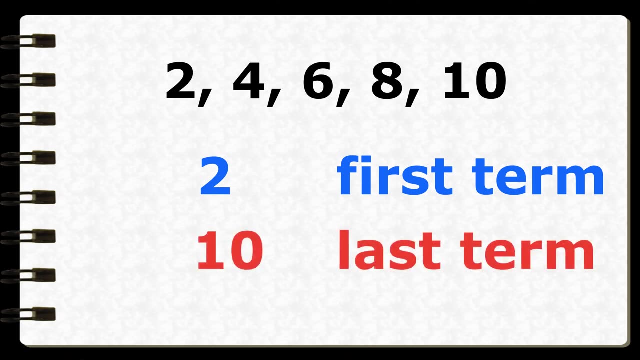 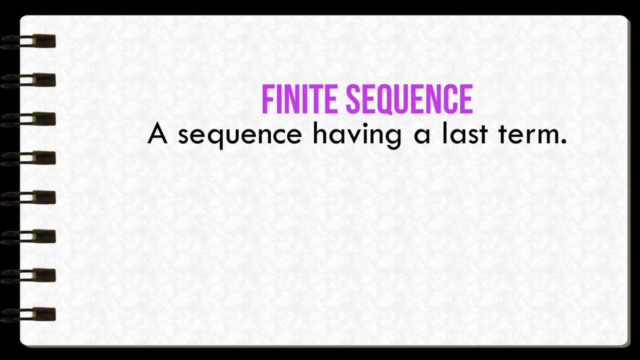 Mathematically it is also called the end term. So let's have this sequence In here: 2 is the first term, 10 is the last term. Get it Okay now. a sequence having a last term is called a finite sequence. 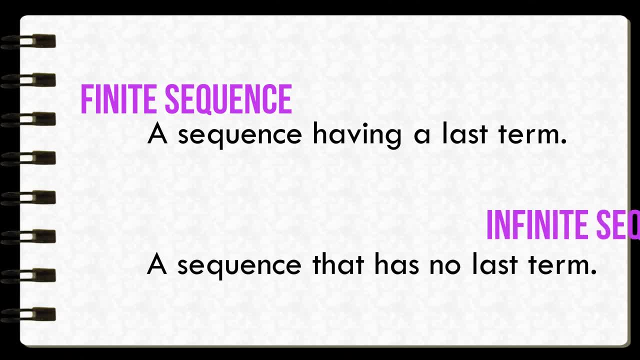 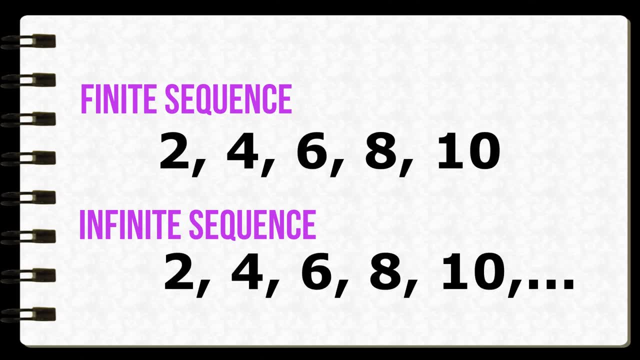 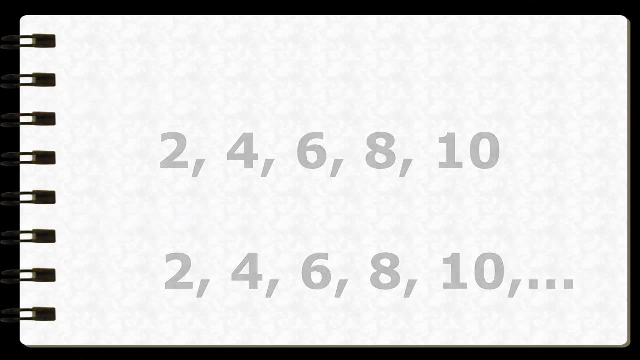 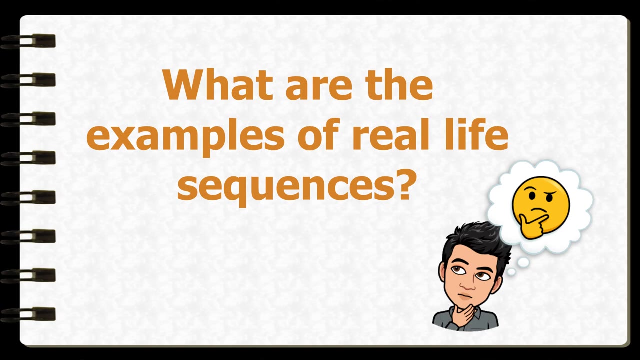 A sequence that has no last term is called an infinite sequence. Let's have these examples. Can you guess what's the difference? That's right, We put this symbol to indicate that the sequence is infinite or endless. What are the examples of real-life sequences? 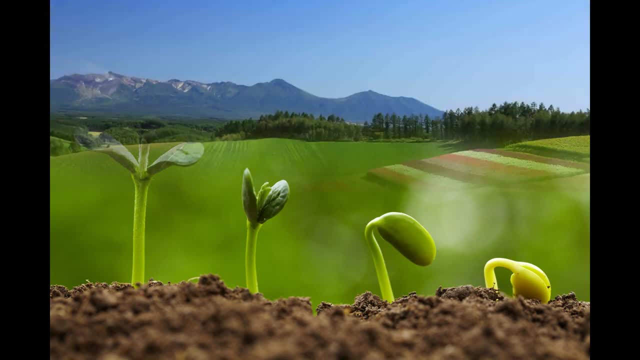 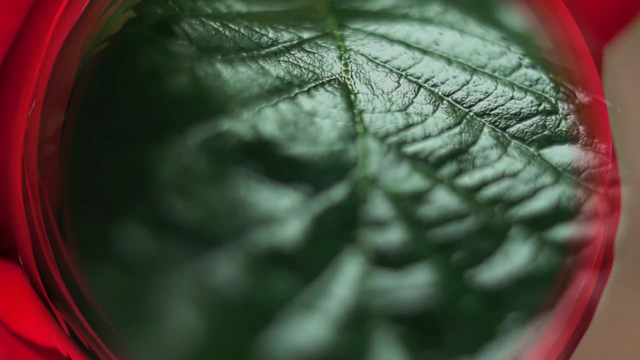 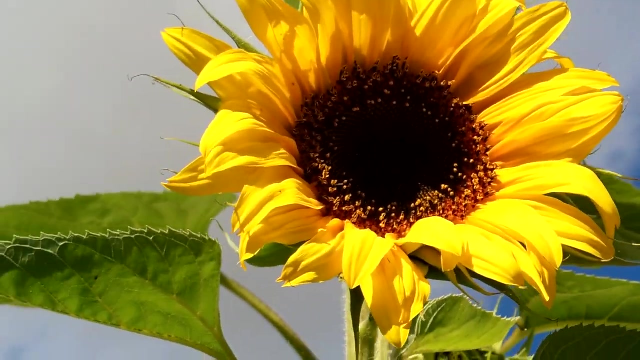 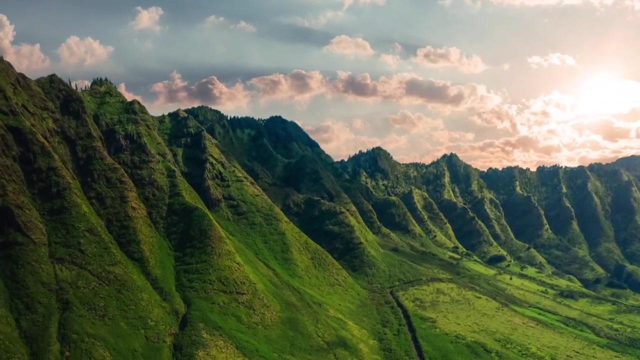 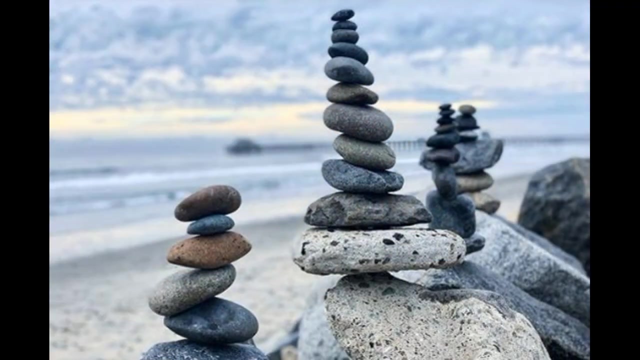 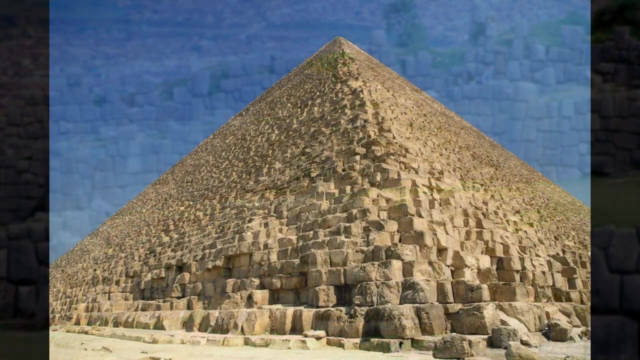 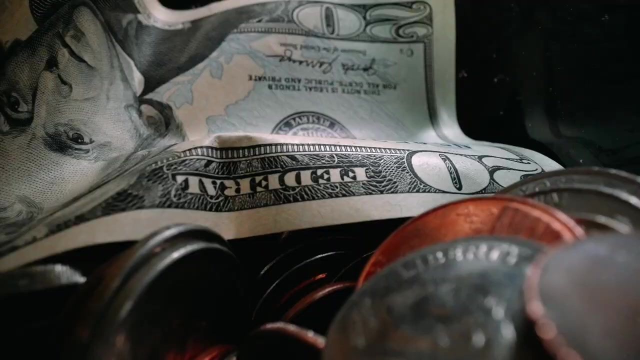 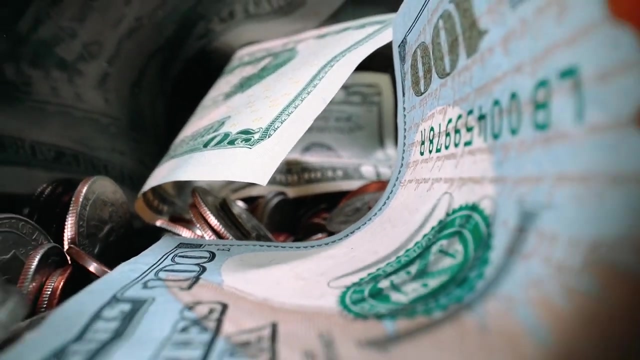 Plant growth, Gardening, Rose petals, Leaf patterns, Sunflower, Mountain ranges, A seashell Stock of rocks, Even ancient structures, The Great Pyramids. Sequences are also used to predict population growth, Doing your savings, Or even solving crimes or mysteries. 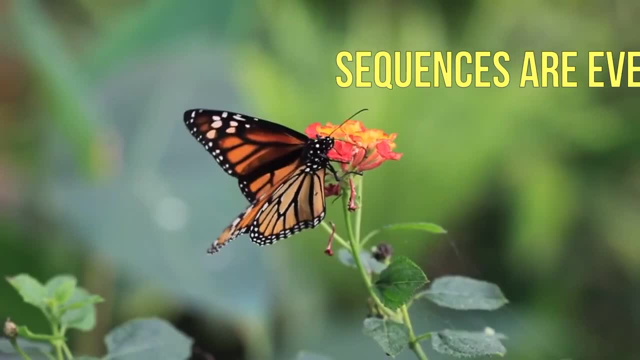 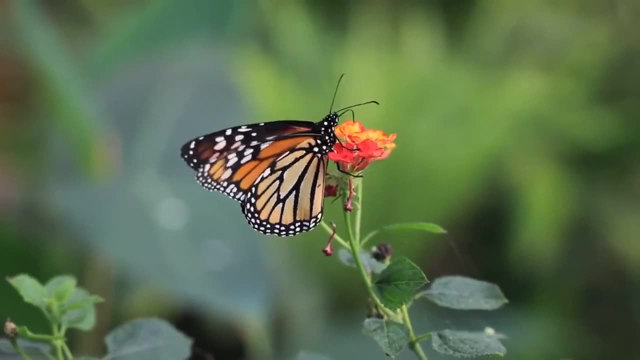 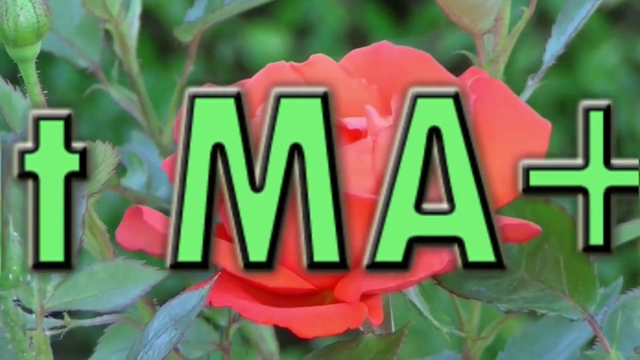 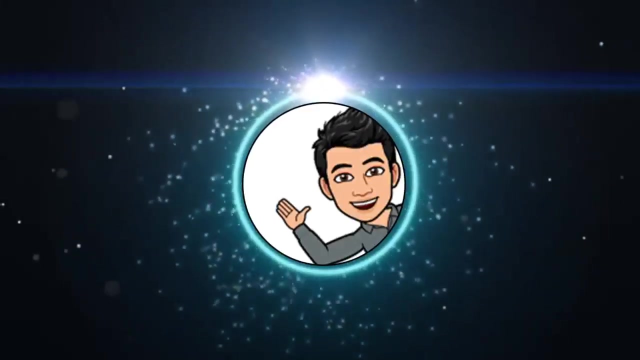 As you know, sequences are everywhere, Because in here we are considering what matters. If you want more videos, subscribe for more.